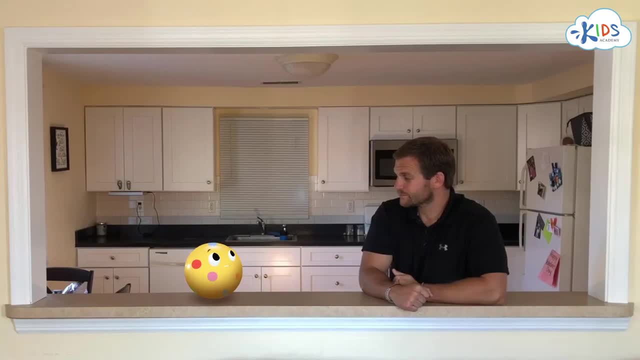 That's strange. All those things are very different. Rain is wet, snowflakes are light and soft and hail is hard and heavy. Are they all really made out of water? Yes, Polly, That's how it is. Like many other materials, water can take on three distinct forms: A solid, a liquid or a gas. 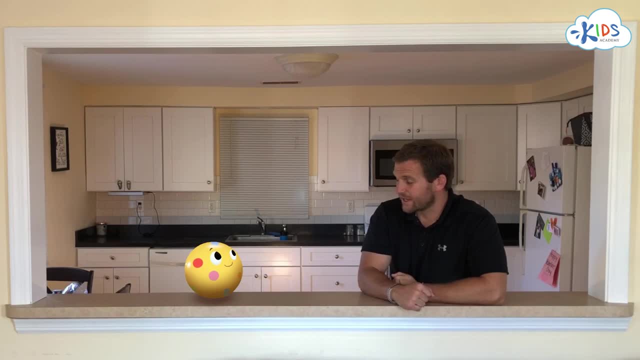 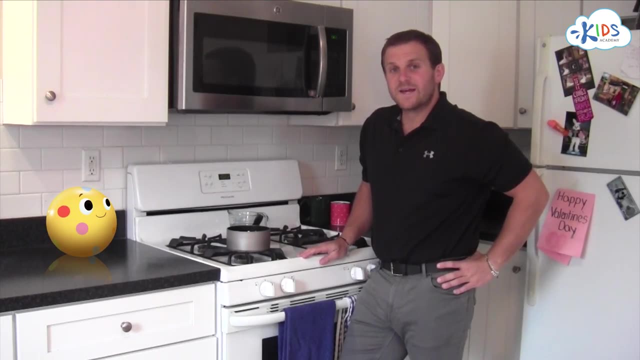 How is that possible? You see it every day. You've probably just never noticed it before. Let's step into the kitchen and take a look. Solids, liquids and gases can be found all over the place, especially in the kitchen. 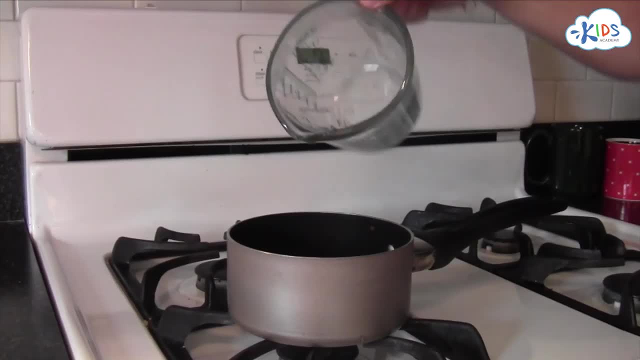 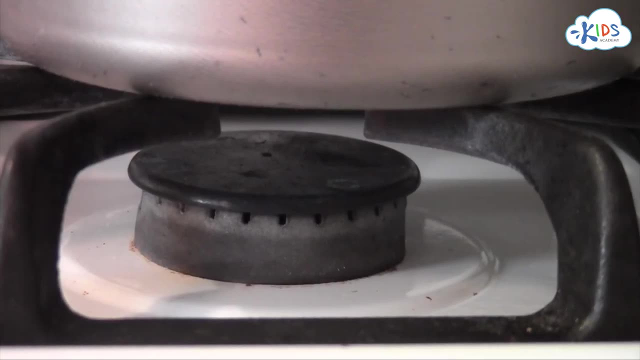 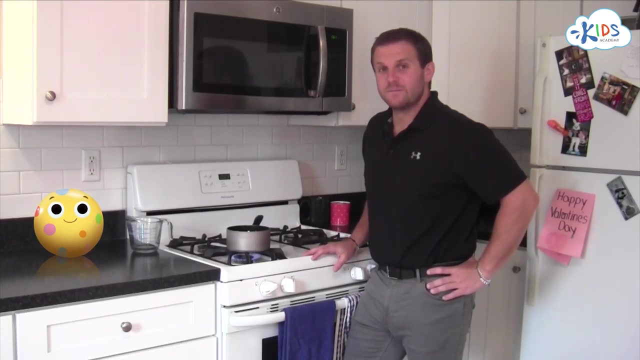 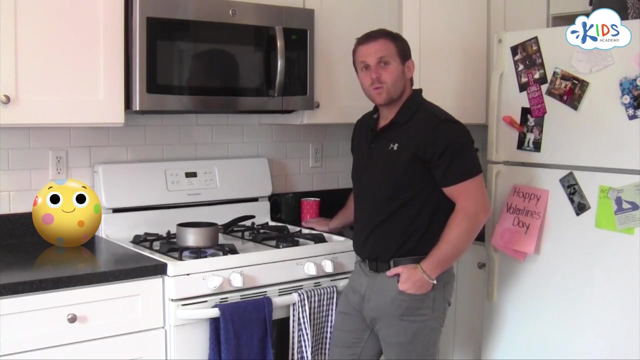 First thing I'm going to do is add some water to this pot. Now I'm going to add a little heat energy by turning on the stove. We're going to wait a little while for that water to heat up. When the water heats up, it starts to make steam like this: 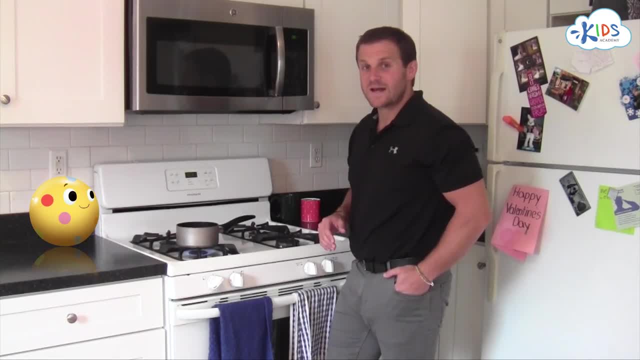 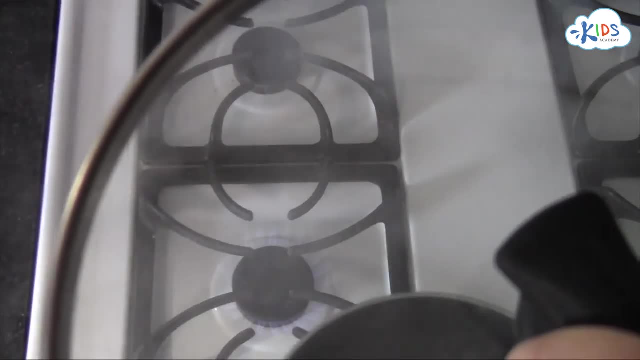 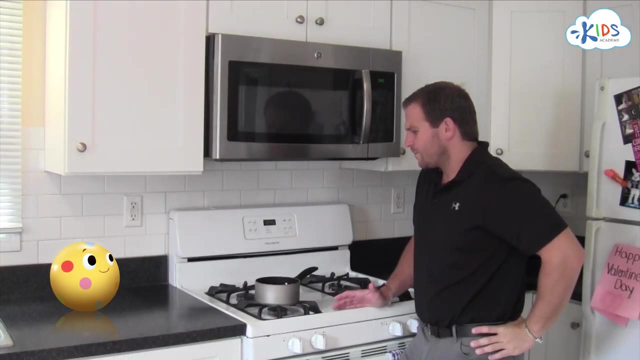 Sometimes you can see that steam collect on things like mirrors and glass. We're going to use a pot top to try and catch some of that steam right now. So, Polly, we saw steam coming out of the pot, but how did we get there? 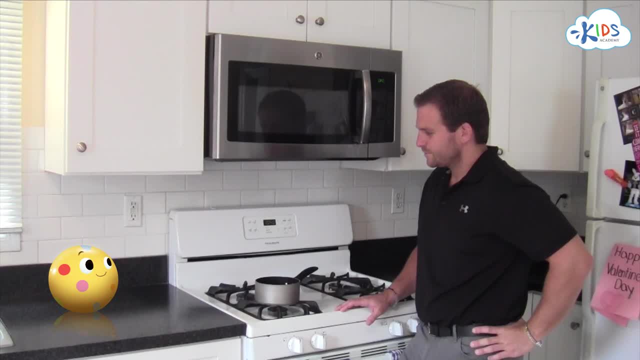 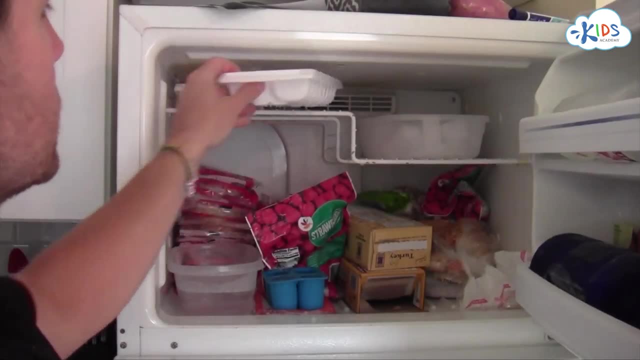 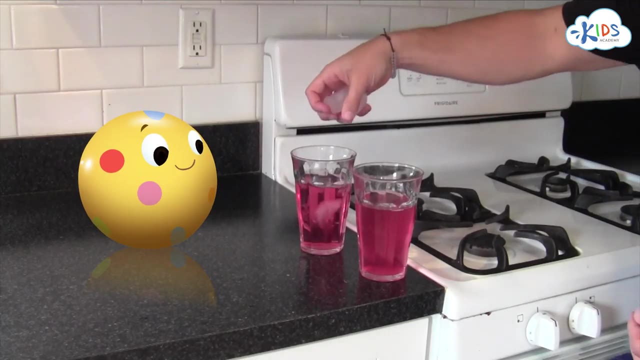 We put nothing but water into the pot. That's a mystery. I've got another mystery for you: How does this ice appear in the ice tray? I know the answer to this riddle: The water's got frozen because it's very cold in the freezer. 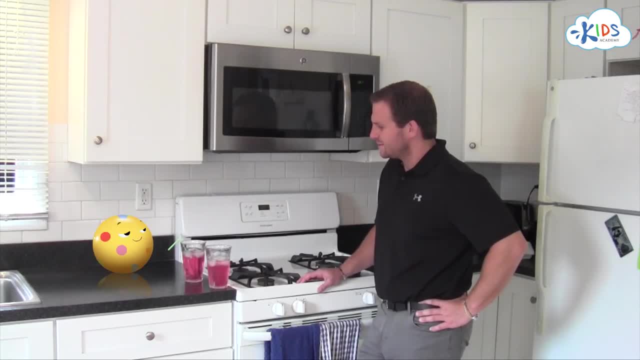 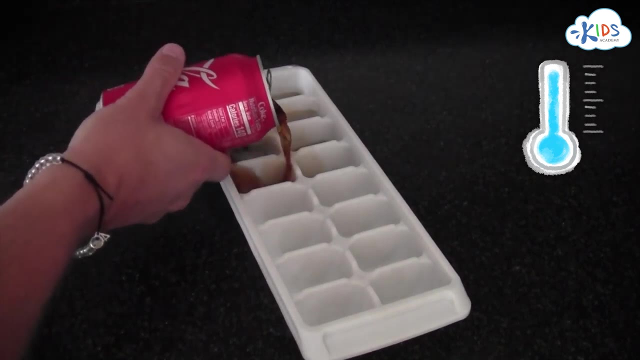 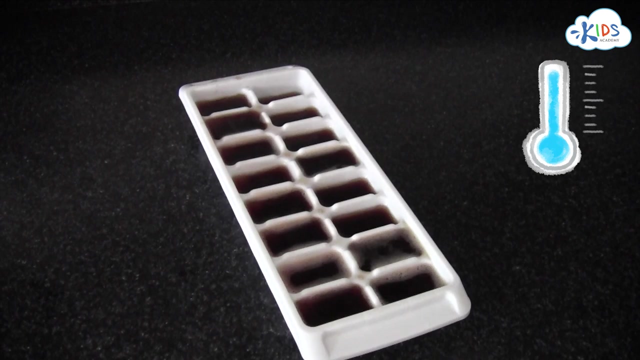 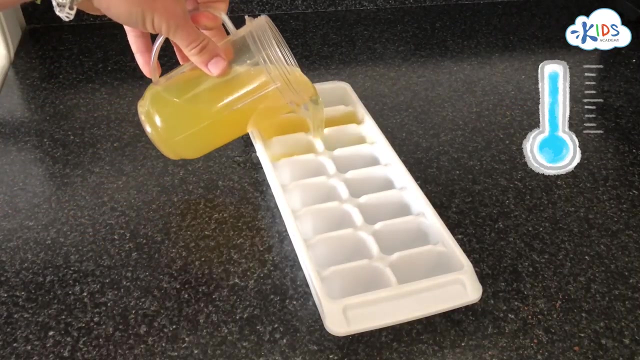 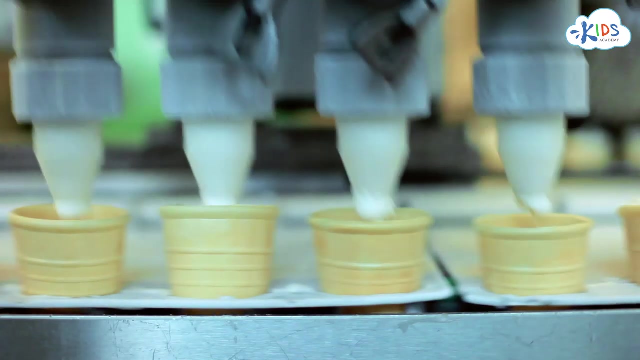 That's right. How'd you guess? I've seen puddles freeze over when it gets cold. Good job. Cooling other liquids down can turn them into solids as well, Like soda Or juice. I love ice cream. If we freeze a special type of milk, we'll get ice cream. 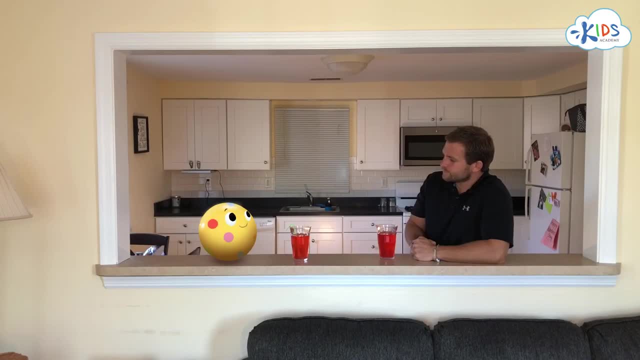 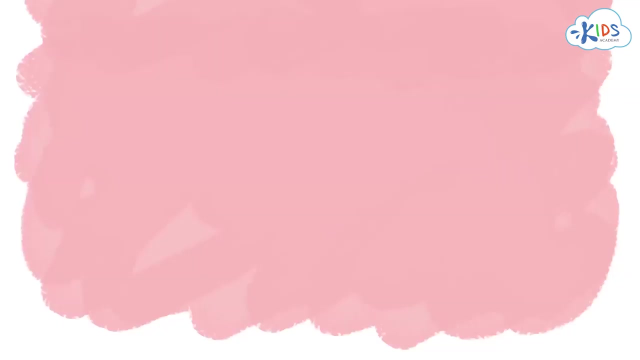 Do you like ice cream Polly? Of course, Especially in summer, I love it. Now I understand what cooling does to liquids, But what about steam? How is it made? When a lot of heat energy is applied to water, it boils and turns into steam. 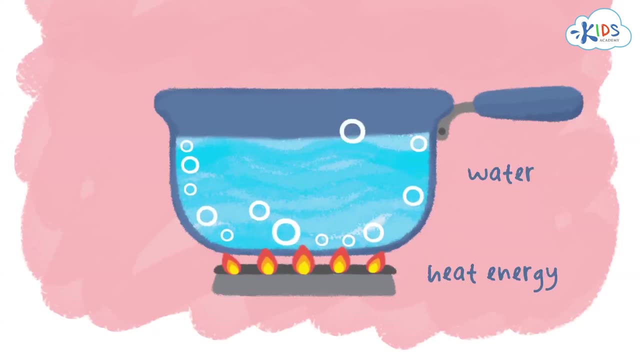 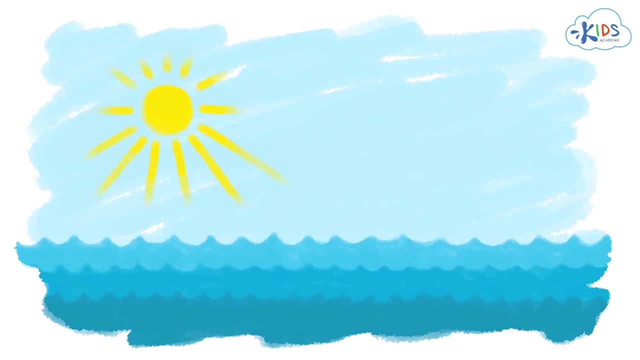 Steam. Steam is very light. That's why it goes up. That means water changes its state from liquid to gas when heated. When a water body like a sea or an ocean is warmed by the sun, the water from its surface turns into light vapor. 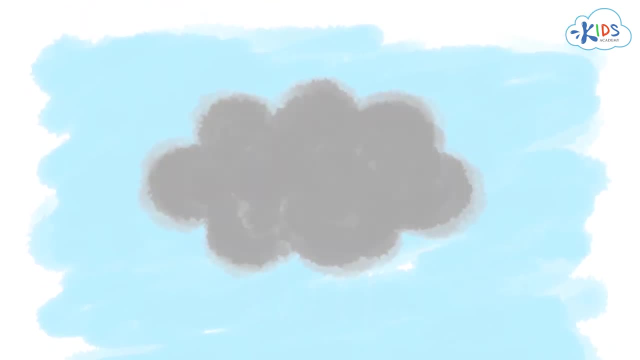 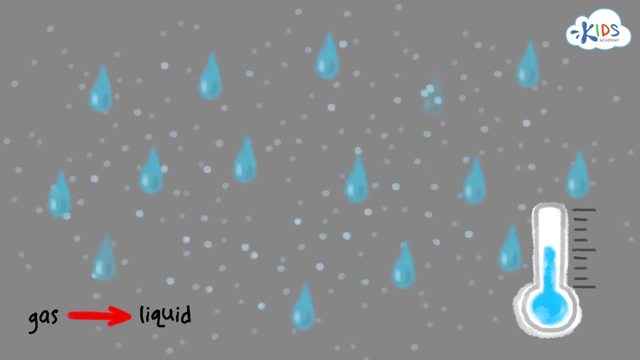 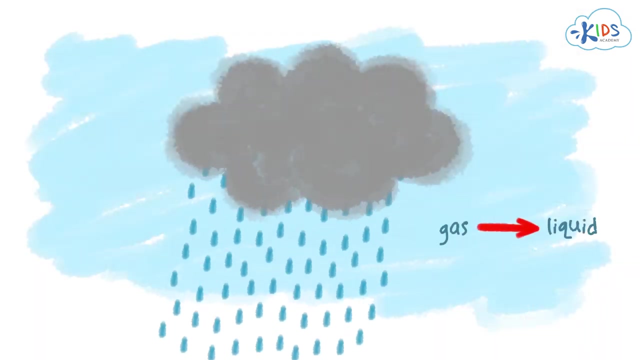 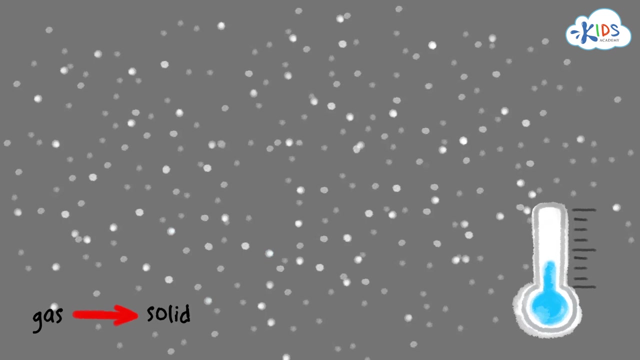 That vapor goes high up in the sky and forms clouds High above the Earth. it's much colder. Cooling turns water vapor back into liquid water that falls down as rain, And if it's winter outside, Then it snows. When it's too cold, water vapor quickly turns into small crystals that stick together and form snowflakes. 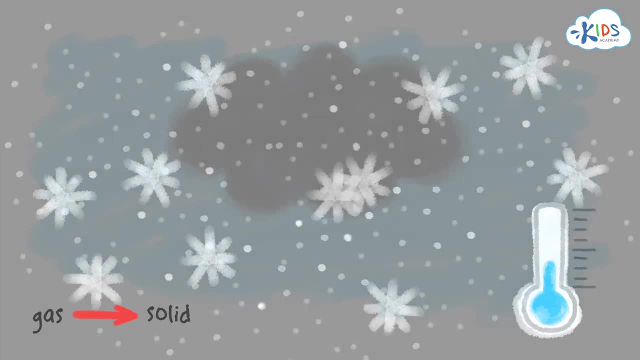 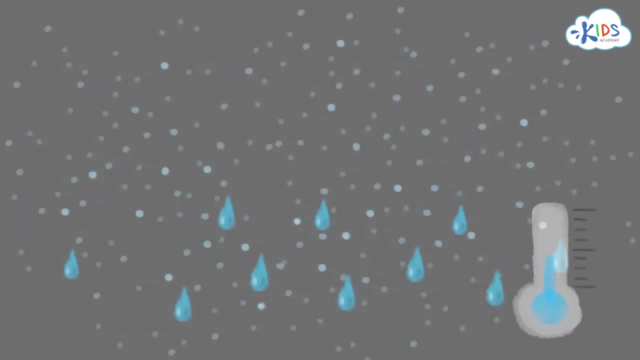 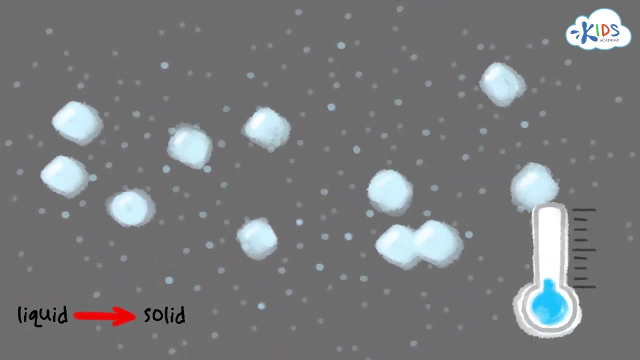 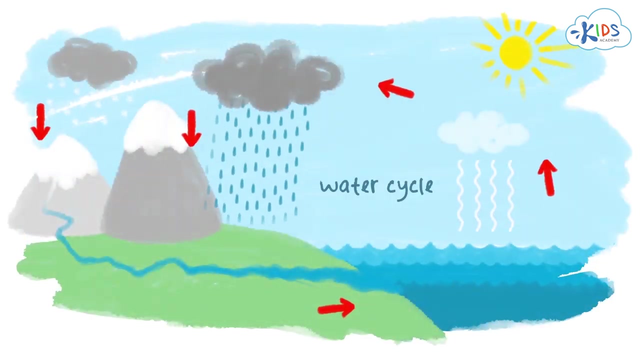 And what about hail? Sometimes, during a thunderstorm, when it's very windy, raindrops in the clouds freeze. They fall down as hail. This is just one of the amazing changes that water can go through when it's heated or cooled.